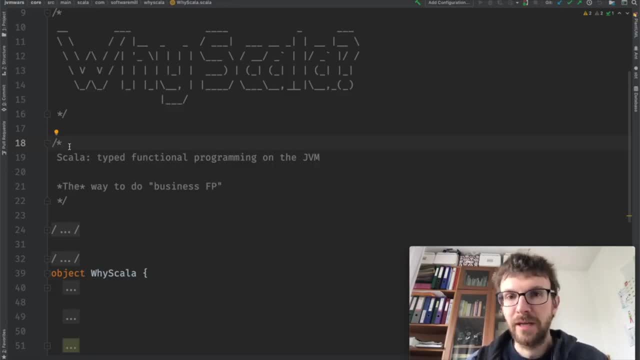 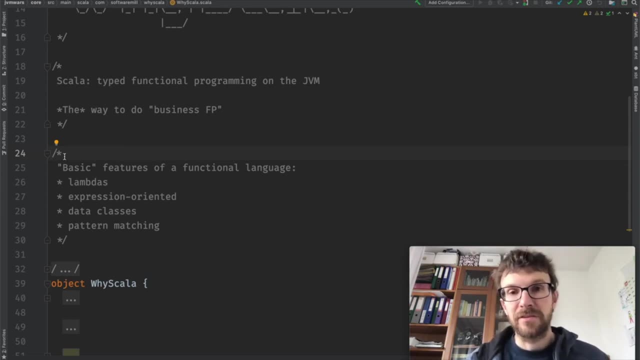 think it is currently the best way to do functional programming in a business setting. So Scala has all of the features, all of the basic features of any program, any functional programming language. So we have lambdas, we have functions which can be treated. 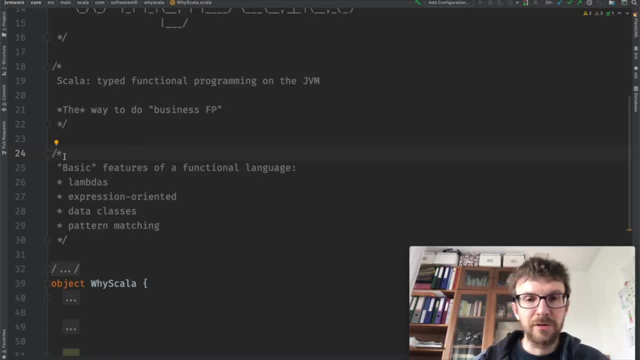 as values. We have methods which can be converted to functions, which are again values, And the whole language is expression oriented. Everything is an expression, And if it's an expression, switch is an expression, and so on. So this is the basis of really of any functional programming. 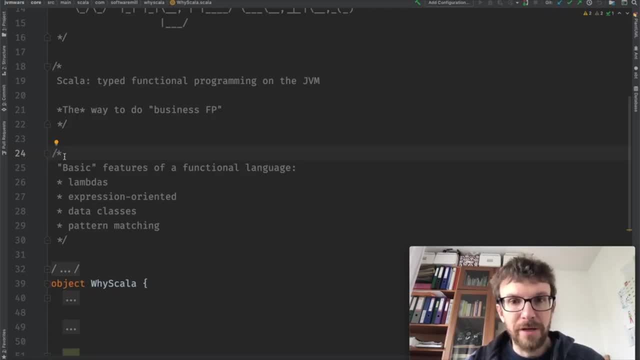 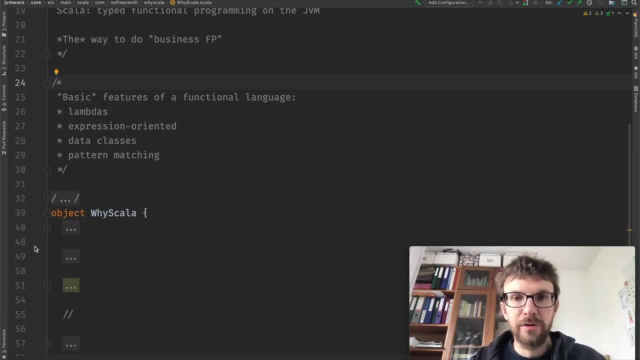 language out there. We have data classes, we have pattern matching, So all of the basics are covered. But what makes Scala unique are some of the more advanced features, some of the features that are not there in other languages, And so, for example, we've got term inference- You might be familiar. 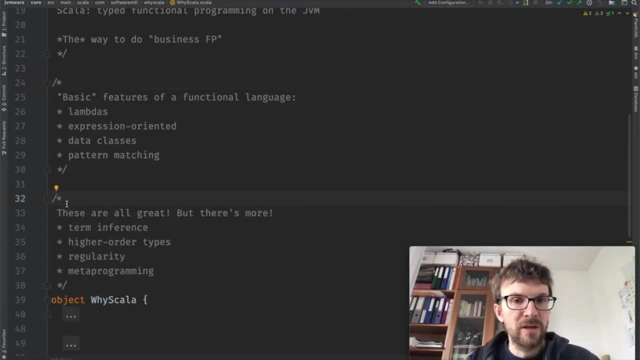 with type inference. So type inference is when the compiler is smart enough to figure out the type of an expression that we have written. Term inference works the other way around: It's when the compiler is smart enough to figure out the expression basing on the type that we have. 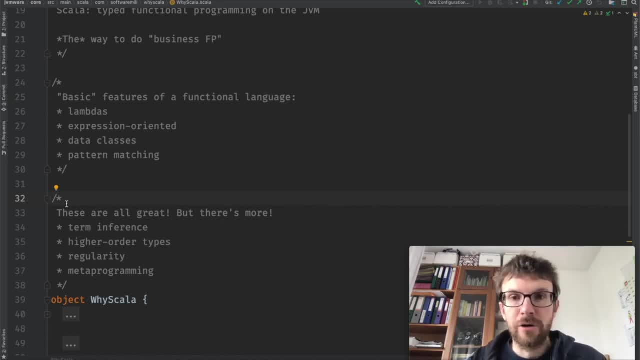 given. So we have a lot of different ways to figure out the type of an expression that we have given. So these are Scala's implicits. We also have higher order types which make it possible to create really elegant, concise and expressive DSLs to manipulate your data. Scala is also a very 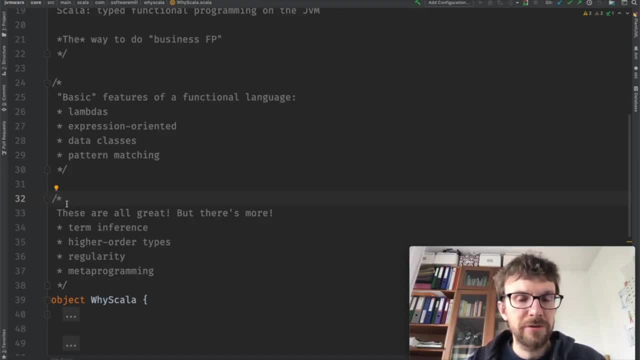 regular language. It doesn't really have that many features, but all of the features it has are very general and they interact in many ways. Some of these combinations of features are really interesting. Some of them are not that interesting, but I think as a community we have learned which combinations to avoid and which to use. 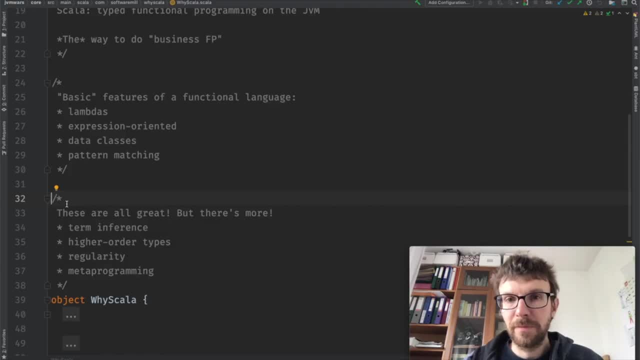 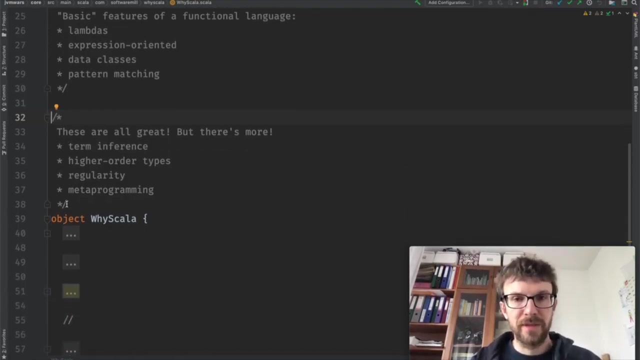 Finally, Scala has quite rich metaprogramming capabilities. Metaprogramming is when you write code which is run at compile time, generates more Scala code, which is then translated into bytecode, JavaScript and so on. But let's look at some specifics. So first of all, 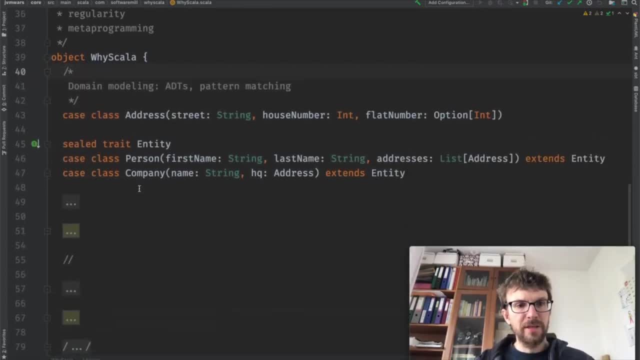 let's look at data modeling. Data modeling is something that we have to do very often, and it's one of the areas where Scala really shines. If you have to model a complex business domain, Scala is a very expressive language and gives you a lot of tools to do that. 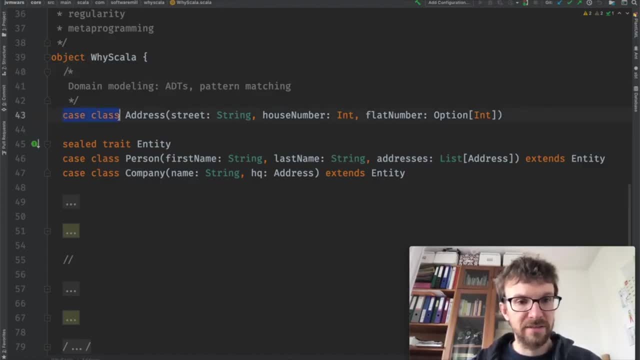 So here we have a case class. A case class is kind of a data class. All of the instances of a case class will be immutable. So once we create an instance we cannot change any data here. So we have a couple of fields. One of them is: 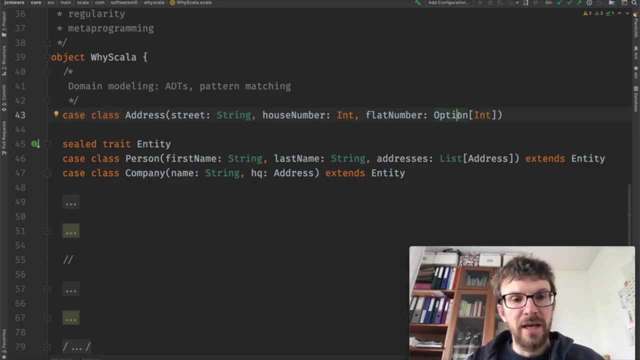 optional. So in Scala we don't really use nulls and null pointer. exceptions and nulls are not really an issue most of the time And that is because everybody uses options. All of the libraries use options to express well optional fields instead of using nulls. So this is a simple 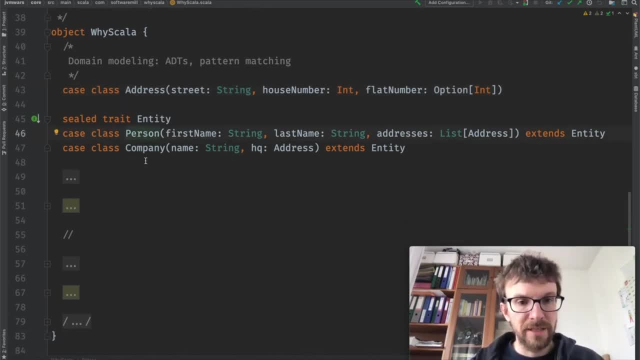 data class. You can also define data classes which form a hierarchy. So here you have an interface, a trade entity which has two implementations. That interface is sealed, meaning that all of the implementations that are possible are enumerated in this source file. So it's either a person or a company, And so this means that if you have an 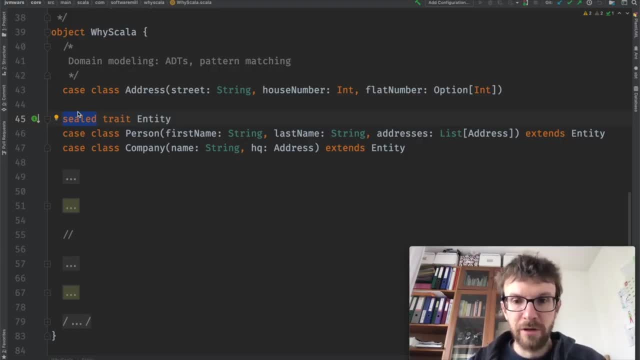 instance of an entity. you can be sure that it's either a person or a company, and the compiler will verify that for you. Here we also have a collection, a list, in this case, of addresses- All of the collections that you are going to be working with by default in Scala. 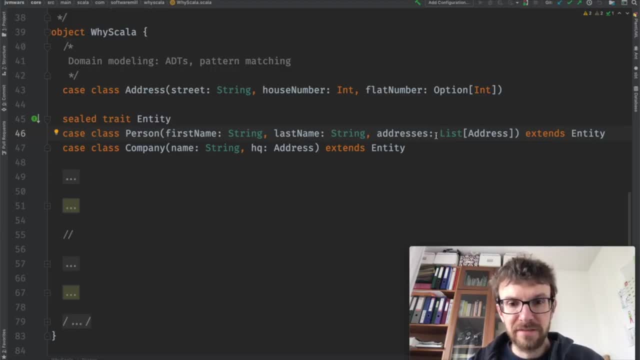 all of them are immutable. So all of the lists, sets, maps and so on- all of these collections are immutable by default as well. This brings us to the first productivity gain, which is that Scala is an immutable first language, and this has deep implications when it comes to 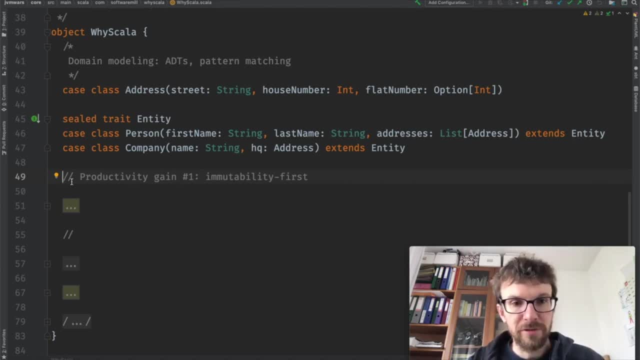 the ecosystem to the libraries. All of the libraries that are written for Scala- and there's quite a lot of them- work predominantly with immutable data structures, with immutable collections and so on, So they form a cohesive whole and they really leverage the 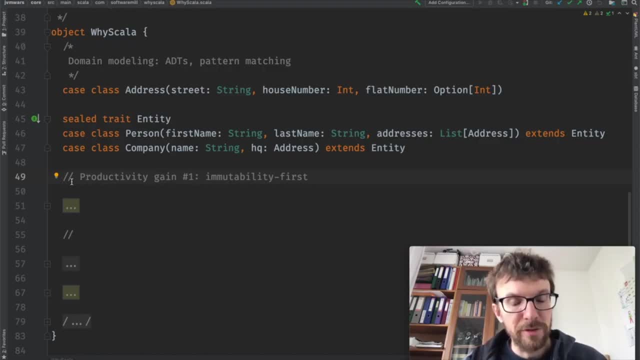 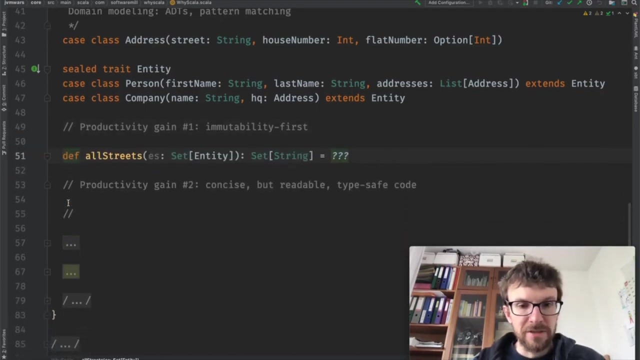 fact that immutability is the preferred way of writing Scala, And this makes things easier to understand and it also makes things partially thread-safe, so you have less problems to worry about. Scala is also very expressive when it comes to manipulating data. so let's say we have a 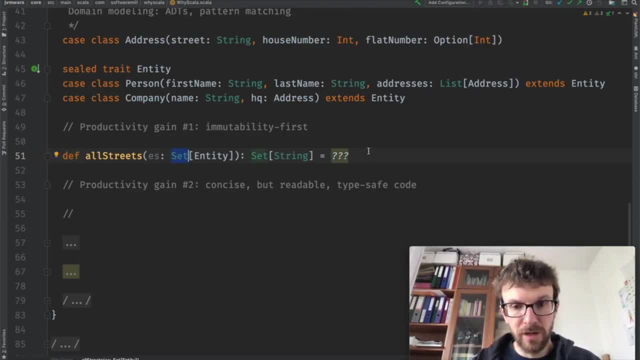 set of streets. so again, this set is immutable. let's say we have a set of entities and we want to extract all of these streets corresponding to these entities. so we take those entities and what we do is we extract first the addresses as a first date. so, as I said, there are two possibilities. 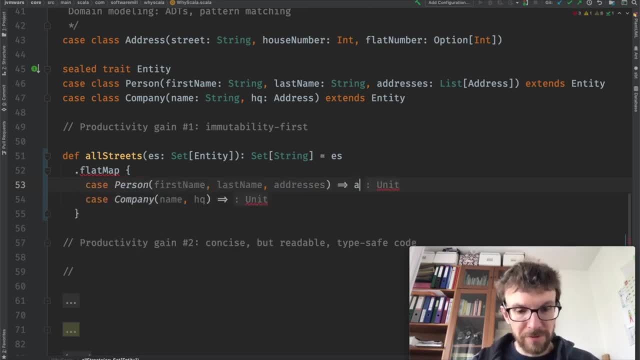 and an entity can be either person or a company. So if it's a person, it's a person, and then it's a document and it's a state, it's a number. so your, we take the addresses, convert the addresses to a set. if it's a company, we create a single element. 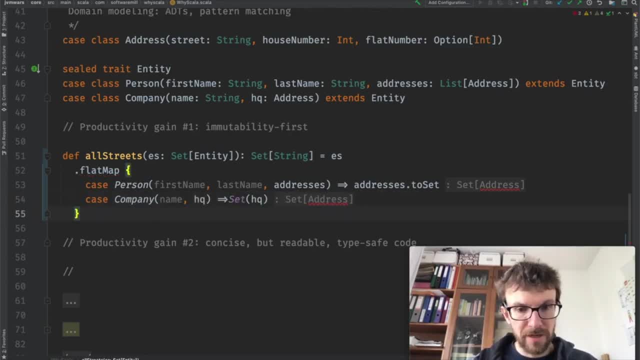 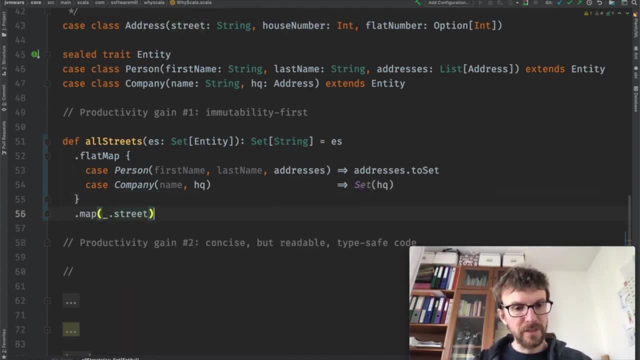 set which is the headquarters of a company. that way we obtain a set of addresses and then we can map this to to the streets and get a set of streets. so this way of manipulating collections and manipulating data is something that's very common in Scala. you're going, you're going to do. 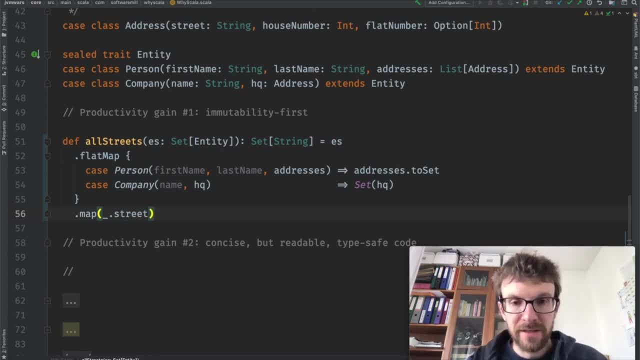 you are going to work with values like this. a lot and a lot of concepts are represented as values in Scala in general- as we will see later as well- and these kind of operations here, where we have been working with an in-memory collection, but they carry over to a more. 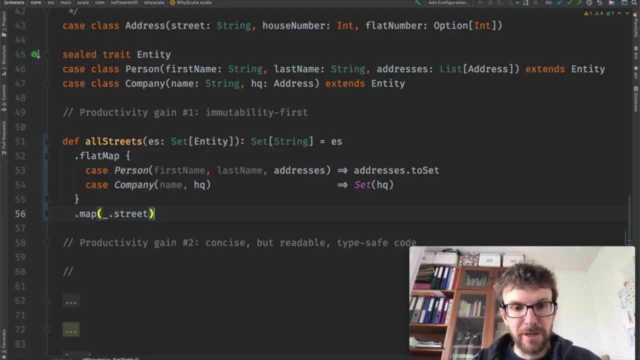 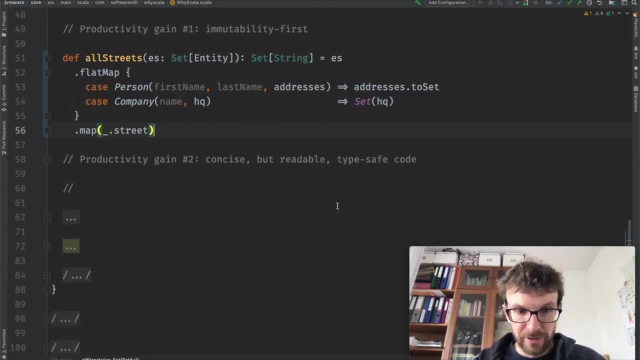 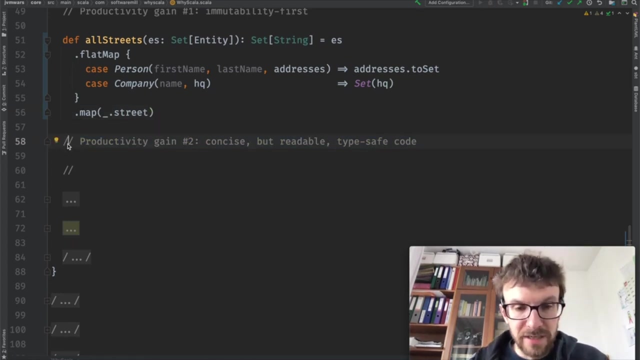 complicated structures as well. so, for example, if you are manipulating a big data set in Spark, the code will look quite similar. this brings us to the second problem, which is the product, again, of Scala, which is that the language allows you to create a concise but still still readable- which i think is very important- and type safe code. so type safe here. 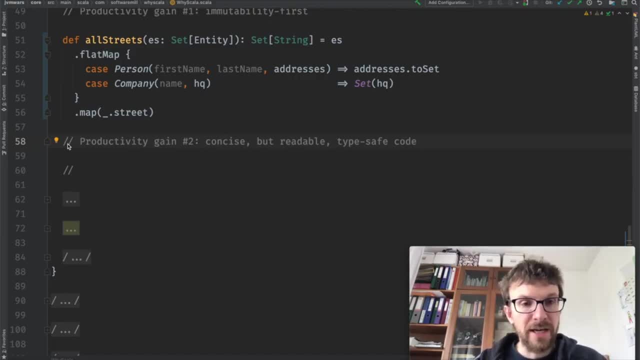 the compiler will actually verify that we can access the properties that that we've written and that, for example, here, that we have covered all of the cases and- and i think the code is concise, it's not really much you can remove from here and, and even if you don't know a lot of Scala, you will probably more or less understand. 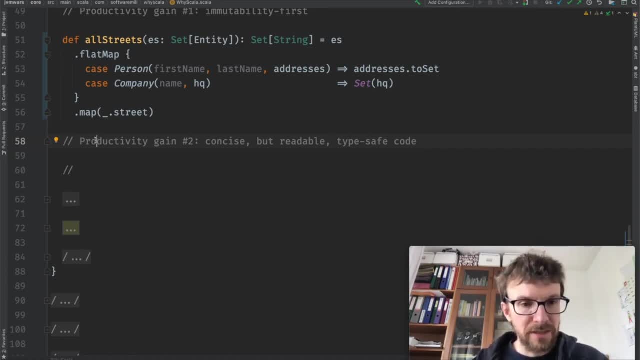 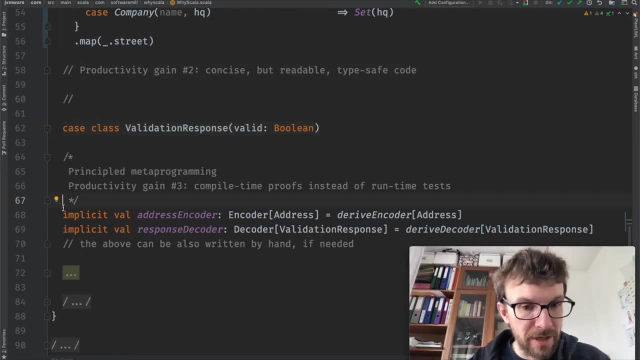 what is happening in that method. but let's, let's carry on. so let's look at some meta programming, which i was talking about in the beginning. so quite often, you know, in in any programming language, we have to do http requests. and when doing http requests, well, 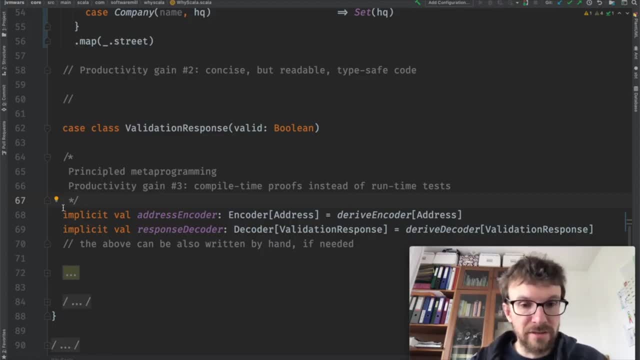 we have to serialize data to json and deserialize it from json and so in other languages libraries and so on. quite often the approach that is taken is introspecting data classes at runtime, for example using reflection, and basing on that doing the serialization and deserialization logic. here the approach is different. what we are going to do is we are 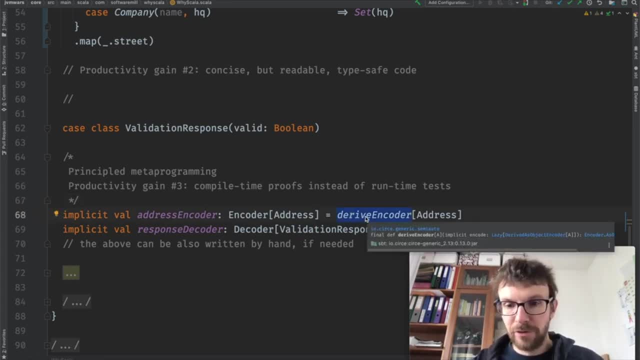 going to use a method which is in fact a macro. a macro is something that runs at compile time, generates Scala code, which is then translated further into bytecode. so this, this macro, over here, it is parameterized with a type, so the type is the, the input for that, for that method, and it will generate code which knows how to serialize an. 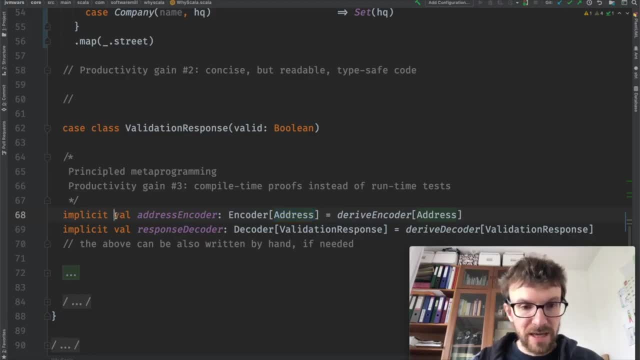 instance of an address into json. so once we have an instance of an encoder, which is really a function from address to json, once we have an instance of that we can be sure that we know how to serialize that class into json properly. so with that said, every compiler in scala component is interested particularly with 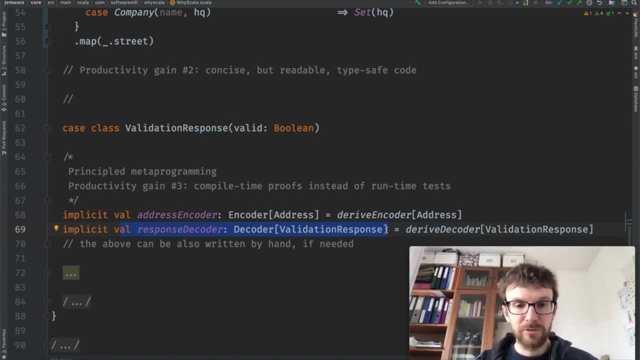 parsing the response. and all of this happens at compile time. and this brings us to the third productivity gain which i wanted to stress over here, is that in Scala we often get compile time proofs instead of runtime tests. so the Scala compiler really verifies a lot of properties for us at compile time. it's true that sometimes it does take some time to. 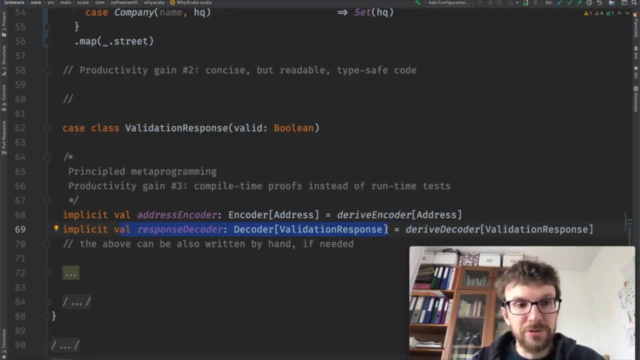 this time for a reason. that is because, well, it actually does quite a lot of work checking that our code is is correct when it comes, when it comes to the types, and quite often, instead of running a simple unit or integration tests multiple times, we can just rely on the compiler to verify a lot. 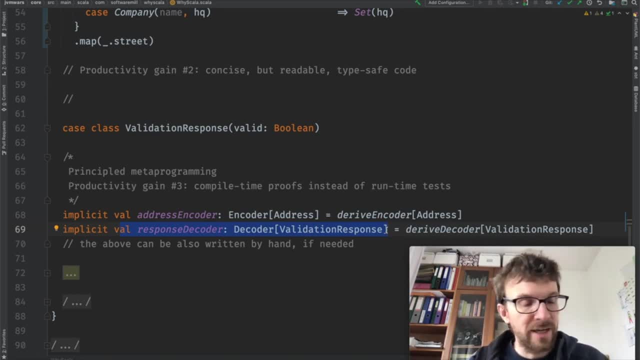 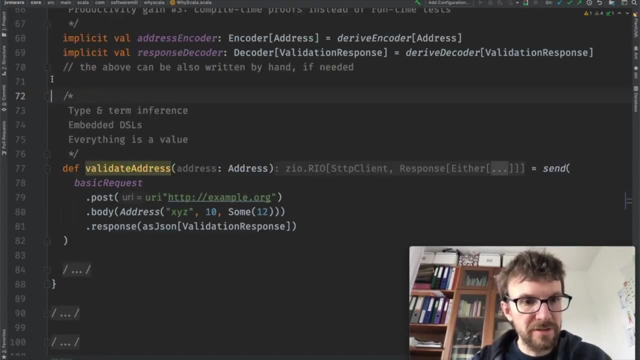 of these basic properties for us and verify on the more and focus on the more complex ones when running the tests. so this brings us to the next example. so here we have an example of how you can send an http request using scala. so what we do is we first describe the http. 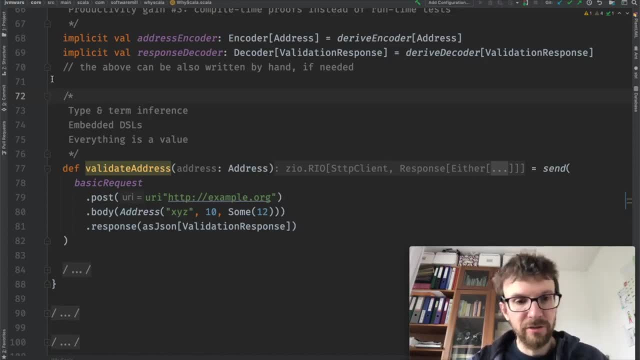 request that we want to send as a value. as i said, we are working with values in scala a lot, so here we are representing the http HTTP request to be sent as a value. can see that there's the address to which the request should be sent, there's the body which to include with the request and also a specification of what to 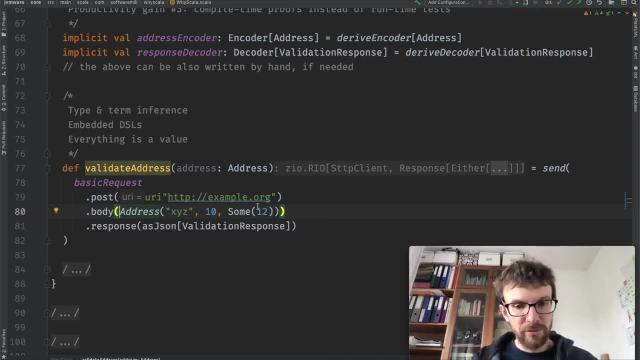 do with the response. so you might note here that, as a body, we are setting an instance of an address. so what the library really needs to know is how to convert this instance of an address into a centralized HTTP body, right? so what it does, what? what it needs? it needs an encoder for this, for. 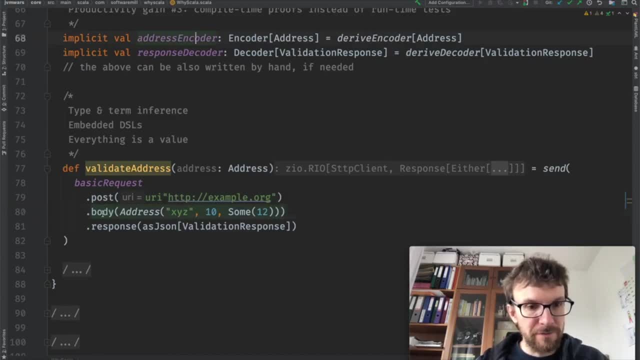 this type, and actually the compiler will figure out this reference here by itself, and this code will not compile if there is, if an encoder for an address is not present, um, in the current scope. and so here we have an example of the term inference that I was mentioning in the beginning. so here, 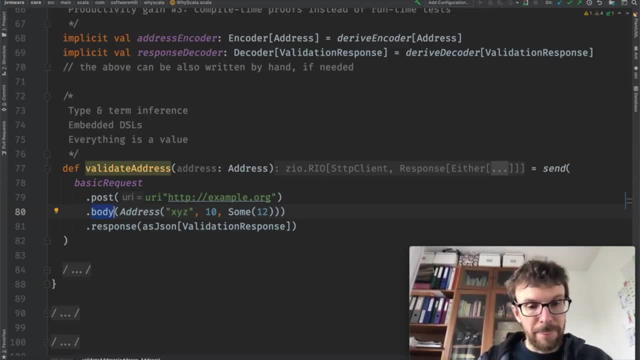 the body method actually requires or looks up an instance given a type. so it needs an encoder for an address type and it looks up an instance, an expression that satisfies the types. same for the response handling over here. so again, if this code compiles, we can once again be sure that we can. 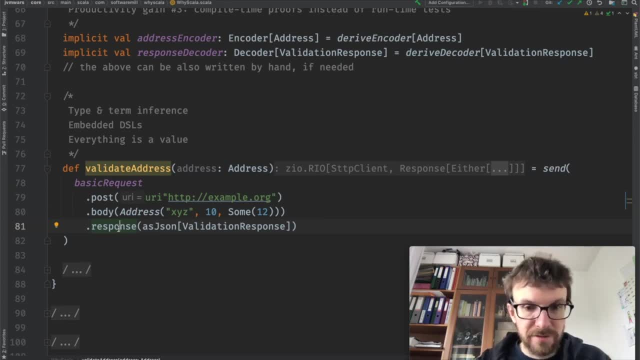 actually send this request and parse the response. so once we have our description of a request ready, which is just a value, we can actually send it using the send function, which you know does all the network stuff that is needed. and this brings us to another productivity gain of Scala that in Scala we are mostly using. 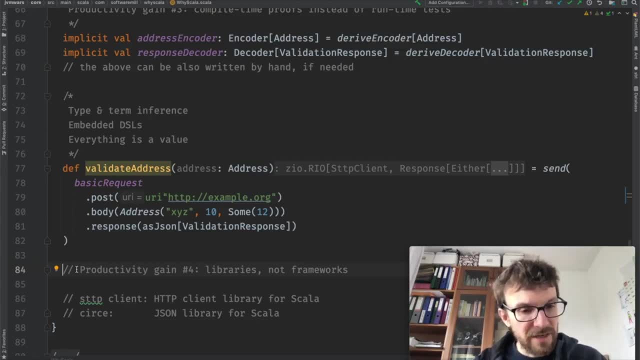 libraries instead of frameworks. so frameworks are very often uh, constraining, uh, while libraries give us a lot of flexibility and freedom. so we don't have to fight the framework anymore, we can use the libraries that work best for our use case. still, it's worth noting that you know libraries. 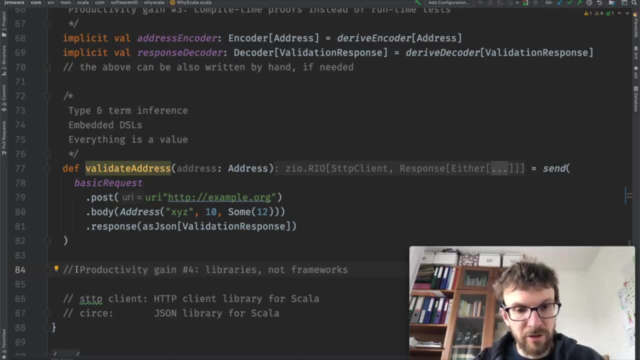 have to form cohesive packages, uh, or they have to work well with each other. so you know you have to work, pick libraries they they also like from their own small ecosystems, but still you get a lot more freedom than comparing to, to using a framework, the two libraries that we've been. 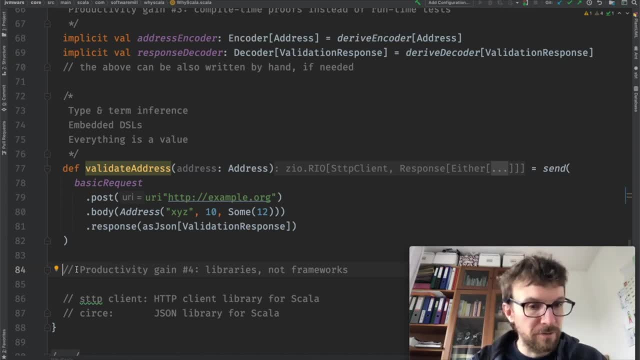 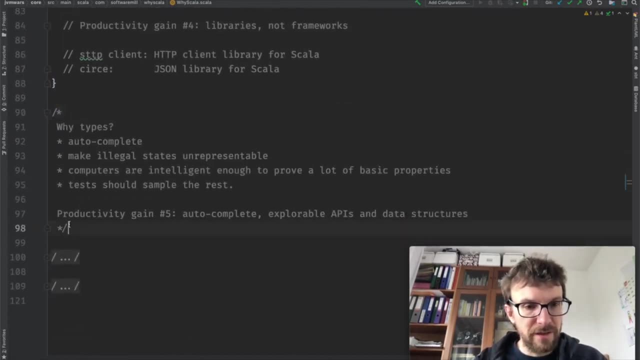 using in this example are http client for HTTP requests and serves you for handling JSON. So, finally, going to the last productivity gain that I would like to mention, Scala really emphasizes types, and the fact that it's a strongly typed language is one of its main features. 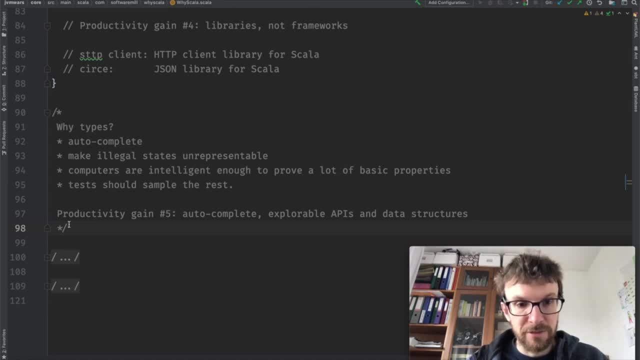 It has an advanced type system. The goal of any type system is to make legal states unrepresentable And I think Scala really pushes the boundary as to how many states or how much you can push, how much you can verify using the type system. 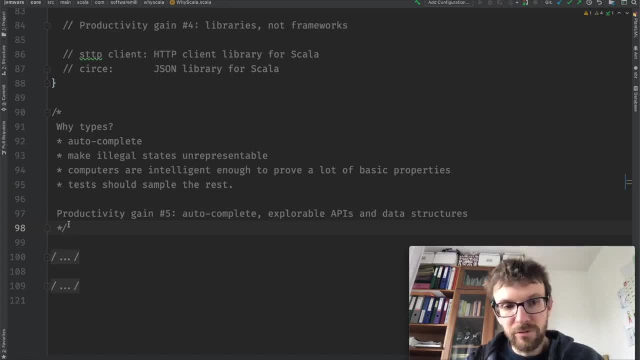 while still being a practical language. Of course there are still some states that will be illegal but unrepresentable, but it's a much smaller fraction comparing to other languages And you know, computers are really intelligent enough to prove a lot of things about our code. 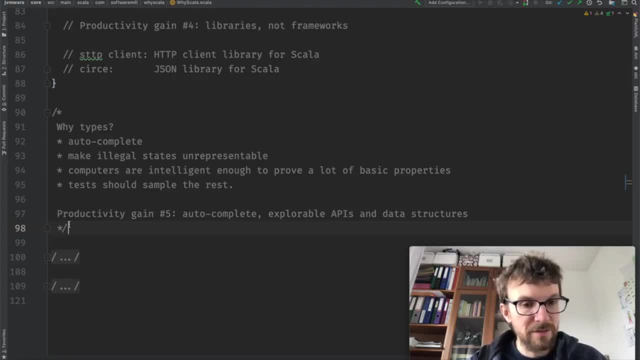 so that we don't have to test it by hand and so that we don't have to fix it by running and repeatedly running these tests. So we can just delegate a lot of this work to the computer, and that's what the Scala compiler does. 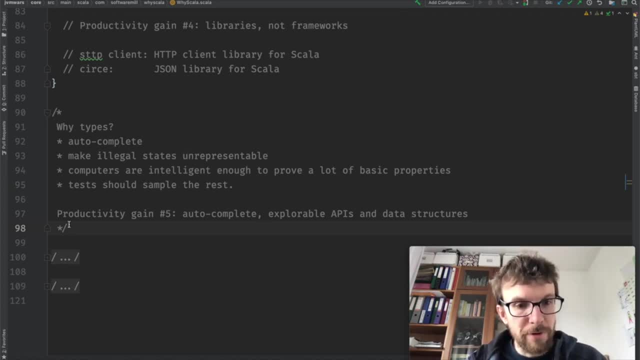 Finally, I think that tests are really a crucial component. not tests, but types are really a crucial component when it comes to the explorability and the way we can understand an existing, a new code base that's well, a code base that is new for us.